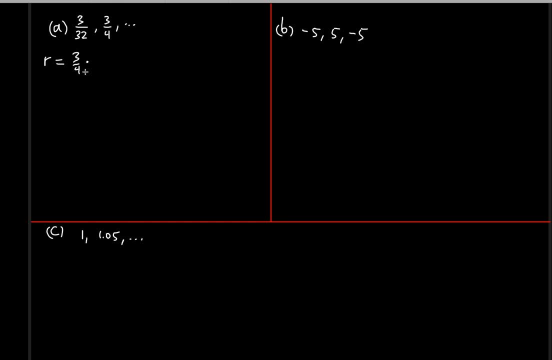 divided by 3, 32nds, And that's the same thing as multiplying the reciprocal of it: 3, 32nds, 32nd, thirds. But as you can see, thirds, threes cancel out, So it's going to be 32 over four. 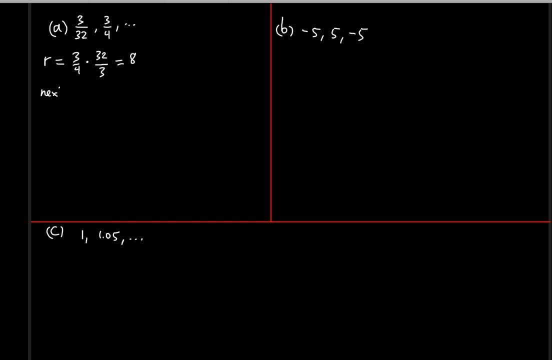 which is eight. So the next three terms should be easy to find. now It's going to be 3, 32 times eight. Well, next three, right? So 3 fourths times eight. right To give us the third term: 3 fourths times eight times eight, right? So basically we're squaring the eight. 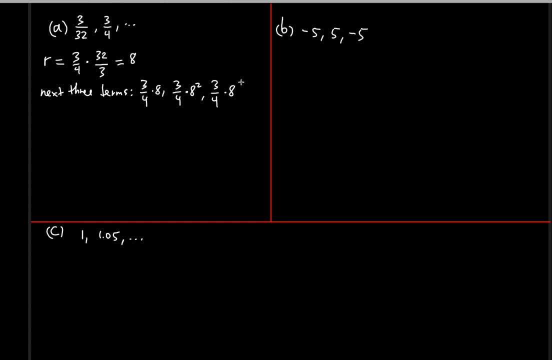 And then we're cubing the eighth for the fifth term. Okay, and this should give you what This should give you. eight over four is two, So that's six. Then this should give you: this should give you two times eight. Sixteen times three is 48.. And this, of course, should. 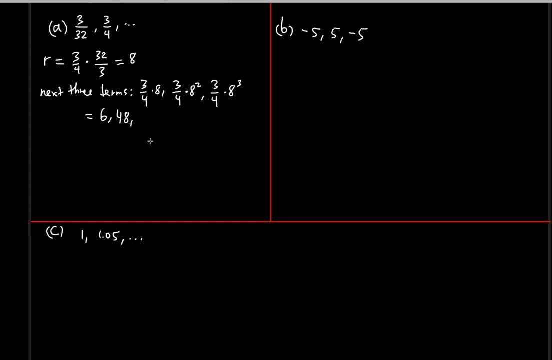 give you 48 times eight, And 48 times eight is 50 times eight minus two times eight. 50 times eight is 400 minus 16.. 400 minus 16 is 384.. And I just did this in my head, I didn't use a calculator, right. 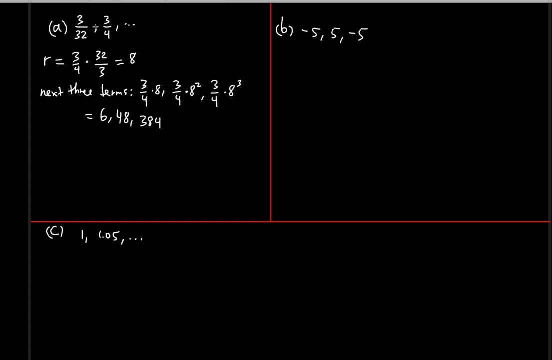 So these are the next terms after these first two: Third term, fourth term, fifth term, respectively. And now, of course, we need to find the nth term formula. So the nth term, we'll just write it as a n. 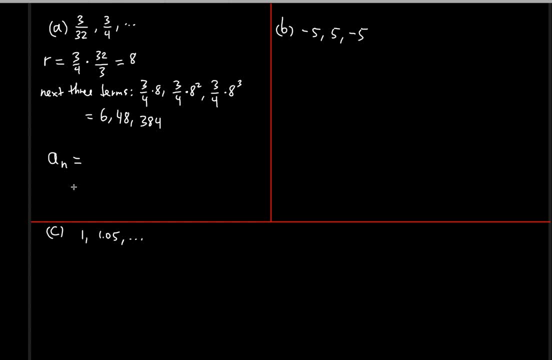 And, of course, when it comes to geometric sequences, we have to understand that we're going to involve the first term, We're going to involve the first term, And then we're going to multiply that by eight. Okay, Now, eight to the. what Eight is going to be multiplied to n minus one in this case? right, Because 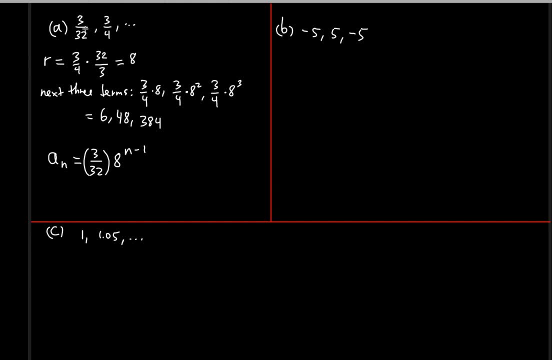 n is equal to. when n is equal to one, we should get this. When n is equal to one, this whole thing is gone, because one minus one is zero. Eight to the zero, power is one. So one times three thirty seconds is three thirty seconds itself, like it should be for the. 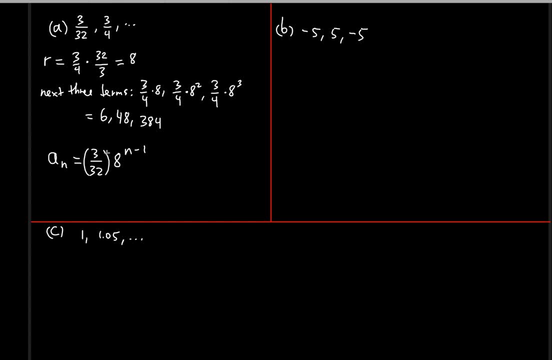 first term. However, I really dislike the look of this. I don't like the fact that we have a fraction here. We can actually work this out. So what I want to do? I want to take the three out And one. thirty twos can be expressed as two to the negative five. Notice that you can. 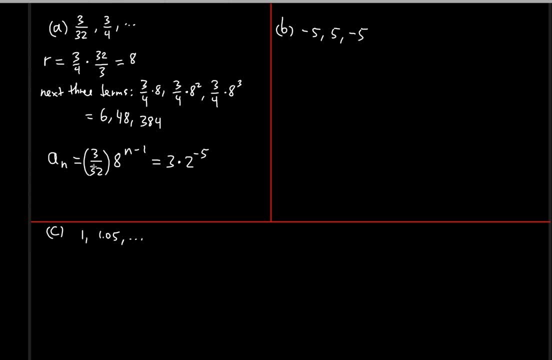 write it this way: Two to the negative five is going to be precisely one, over thirty seconds, because we took the three out. It's already there, And now we can express eight as two to the thirds being raised to power n minus one. Okay, which should give you, if you use your algebra, this should give you what This should. 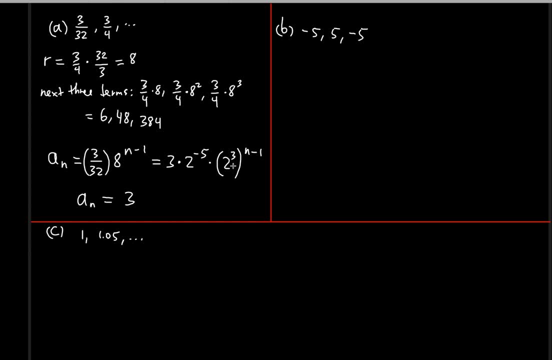 give you three, and then this is what: Two to the three: n minus three minus five. So it's going to be, it's going to be: 2 to the power of 3n minus 3 minus 5 is what 3n minus 8, if you do the algebra. 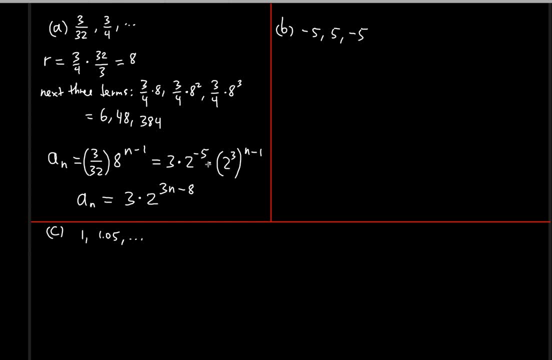 right, you're just going to combine the same bases. before you combine them, of course, you're going to distribute this power 3n minus 3, and then you're going to combine the two bases by basically adding the 3n minus 3 with the minus 5. you should get 3n minus 8 as the single base. 2 right? so I know? 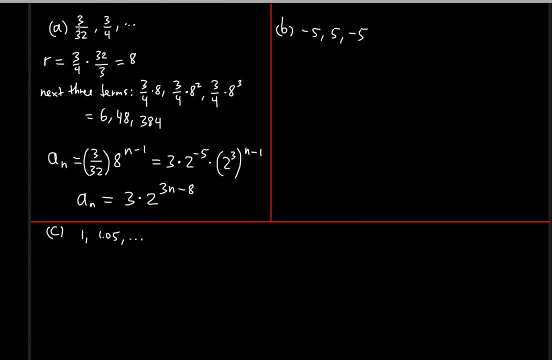 you might say: but this is not the first term, you're going to get 3 32nds, you're going to get 3. no, you're not going to get 3 if you, if you put an n is equal to 1, you're going to get 3 minus 8. 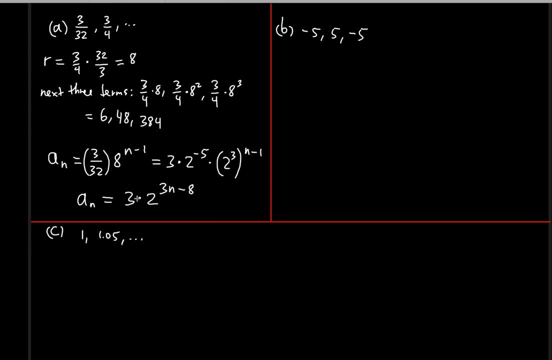 2 to the minus 5 is 1 over 32. so you do get 3 32s for the first term. you don't get 3, so be sure that you understand. the fact that we have a different um power for the two here compensates for the fact that we no longer have a 3- 32. 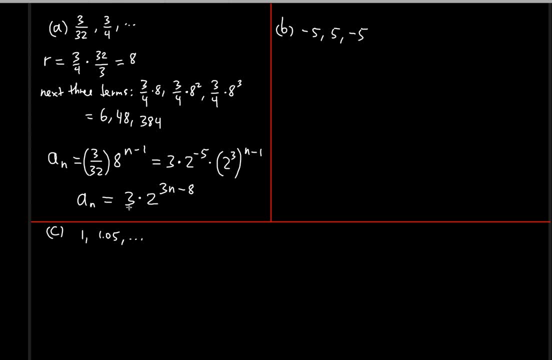 we have a 3 as a seemingly first term, but that's not true. it's not going to be the first term, right? I just like this better. I don't like using the fraction like this, but basically this is equal to that, right? but we can make this look neat, so we just say that this is the nth term formula. 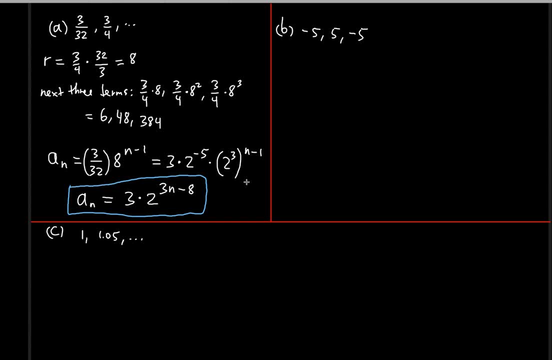 for this sequence, geometric sequence. now the next sequence. that's going to be fairly easy, right? you know the common ratio is going to be minus 1. right 5 divided by negative 5 is not minus 1, or negative 5 divided by 5, same thing minus 1. so the next three terms, that's going. 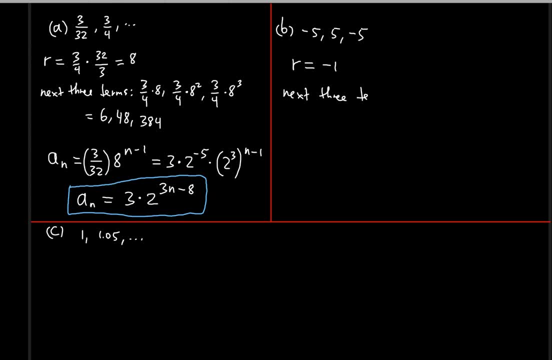 to be easy, right, you just alternate the signs and that's it. you just alternate the signs and let's see. so you alternate the signs, so you should get 5, you should get minus 5 and then you should get 5 again, right? so that should be clear. and just multiply. 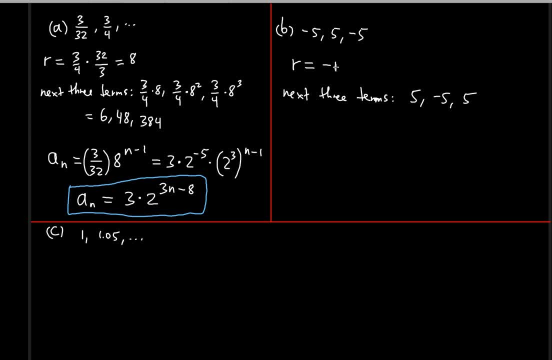 this by negative 1, you get 5. then this by negative 1, again, you get negative 5. this by negative 1, again you get positive. right, that's, that's pretty easy. that's easy to see. so now, how do we find the nth term formula? you realize, of course, that 5 can be taken out. 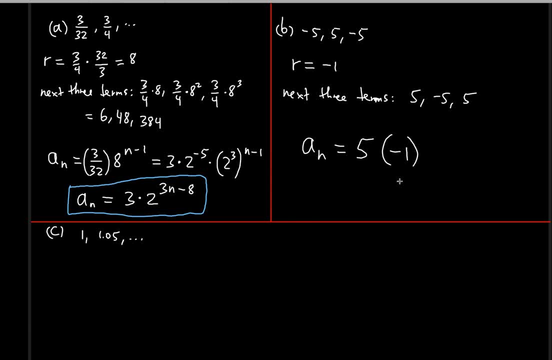 and the negative 1 will be played around with how, when n is equal to 1, if we put n here, is that going to work? when n is equal to 1, this should be negative because the odd power for the negative number gives you still the negative, and it's good because the first term should be negative. 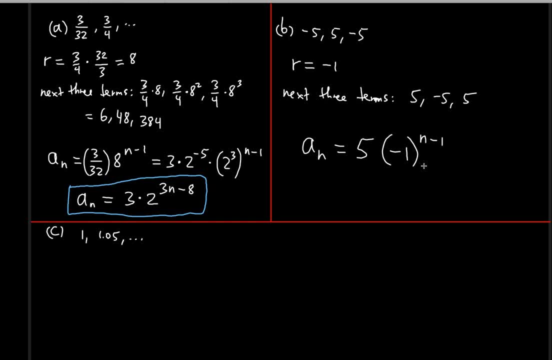 right. so you're not going to write n minus 1. n minus 1 will be false because that would. when n is equal to 1, you would get a positive right minus 1 to the 0. power is positive, but you should have a negative number, negative 5 right. so minus 1 is not necessary. this will be the correct. 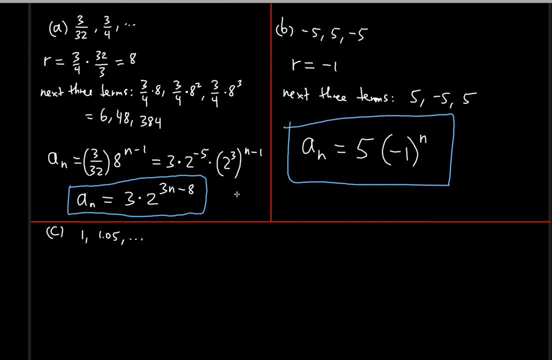 representation of the nth term formula. now, lastly, here the r value first is going to be the quotient of the next term by the preceding term, right? so 1.05 divided by 1: 1.05, good, so the ratio seems to be the same as the second term. that's good. so the next three terms next. 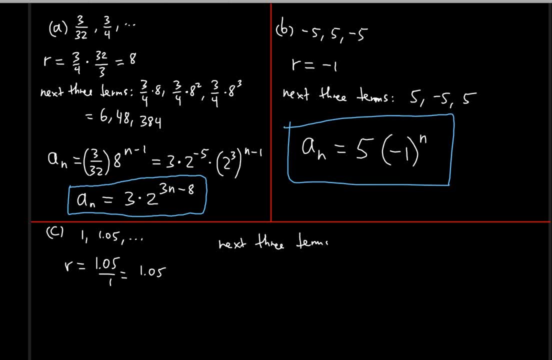 three terms. next three terms will be what 1.05 times the ratio times itself. so we're going to square that. as you might have guessed, the next one will be cubed, because you always multiply it by 1.05, whatever the preceding term was 1.05 quadrupled, so that's easy. so now the nth term formula is: 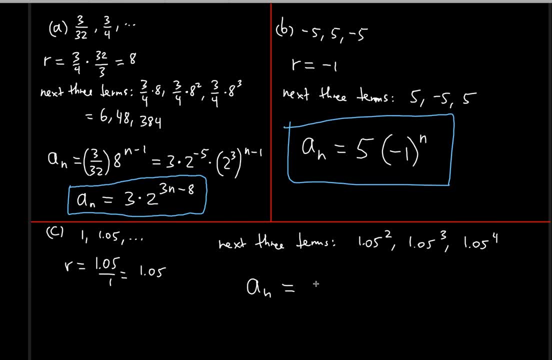 easy as well, pretty easy, right? so you just write, of course, 1.05. and remember, we can write 1 outside, of course. but if you write 1 outside, it's like not writing it at all. right, you can just write. you don't have to write 1, because we know that the number always 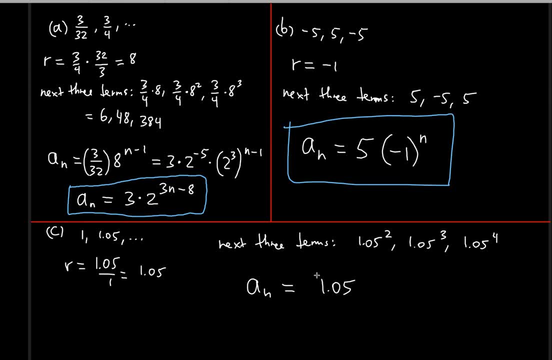 all always multiplies by 1 to give itself right, so just write parentheses. now we, we got to transform this into a 1 when n is equal to 1. so if we, if we put, if we just put n, it's not sufficient, because when n is equal to 1, this is this: gives you 1.05 for the. 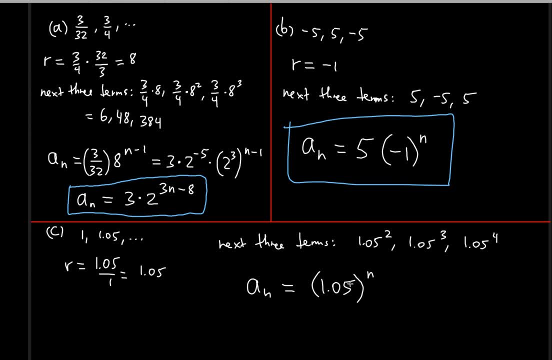 first term. but the first term should be 1, not 1.05. so you should subtract 1 so that when n is equal to 1, you get 0 for the power. 1.05 to the 0 power is 1. when n is equal to 2, you get 2 minus 1 for. 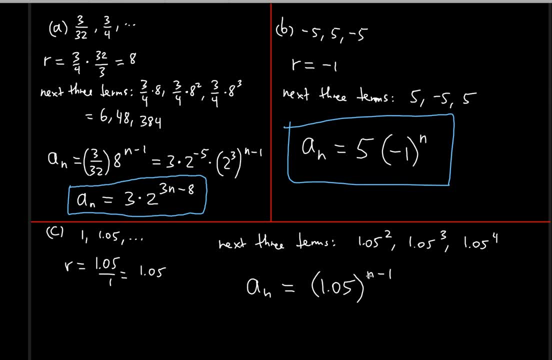 the power. so you get 1 as the resulting power. 1.05 to the first power, when n is equal to 2, gives you precisely 1.05, and so on and so on. for the next terms, right, and here will be 3, the. 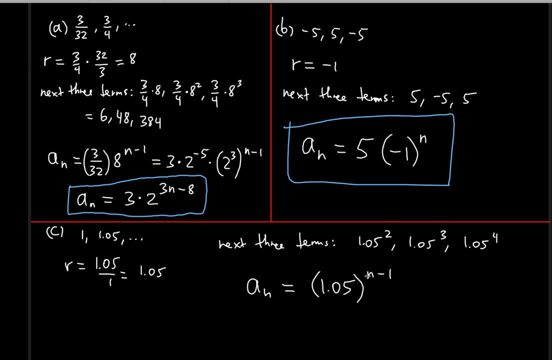 resulting power is 2, as it should be. n here is 4. 4 minus 1 is 3- beautiful- and n values 5 for the fifth term. this will be the fifth term, precisely 5 minus 1, 4 power. all right, so I hope this was uh useful. thank you so much for watching and see you in the next video. foreign. 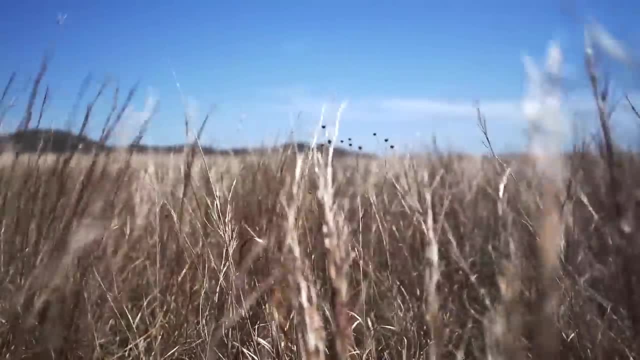 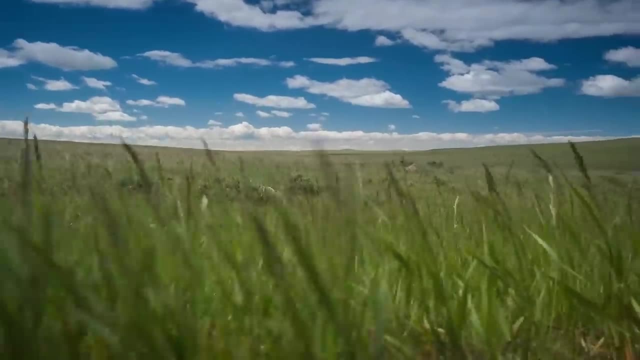 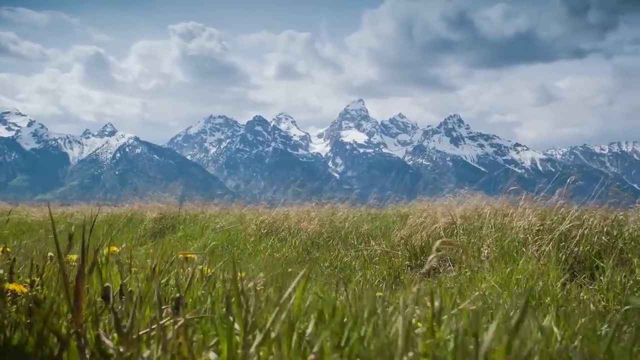 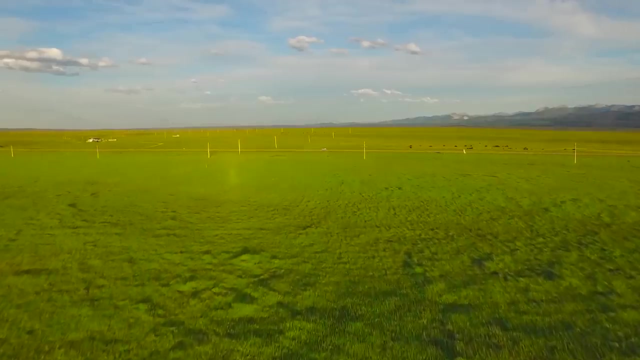 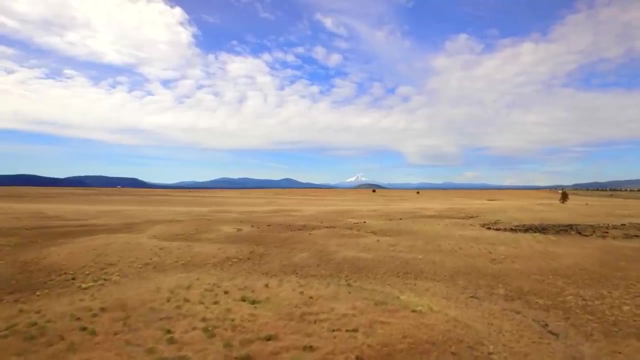 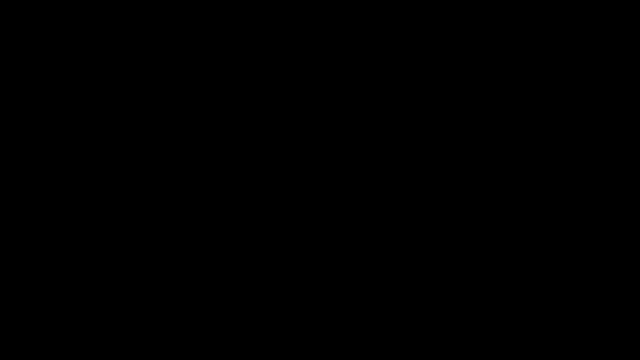 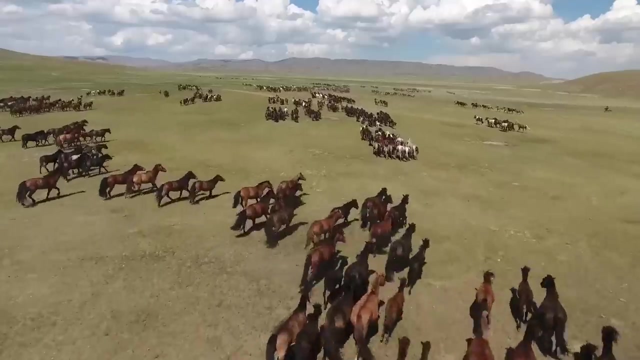 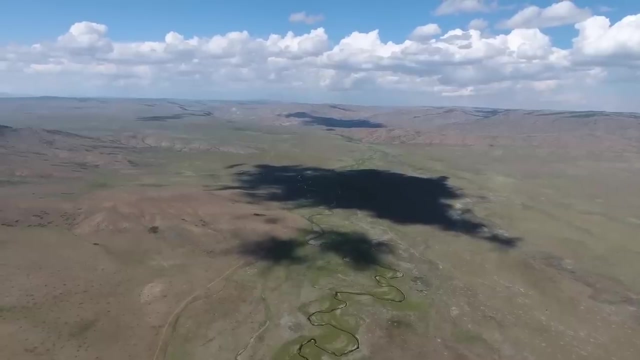 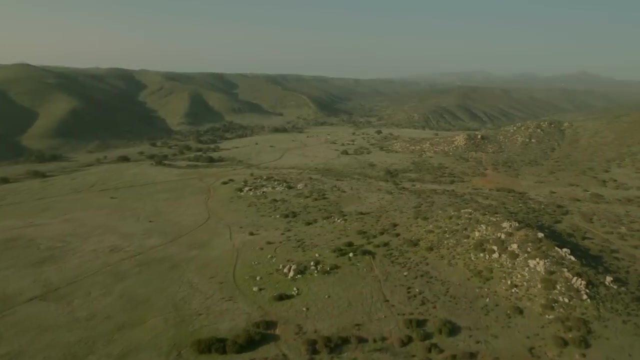 Please leave a comment. Please call 706-950-7000.. Please leave a comment. Please leave a comment, Thank you. If there is one plant that has come to dominate our world, it's this, Occupying every biome on Earth except the ice sheets. 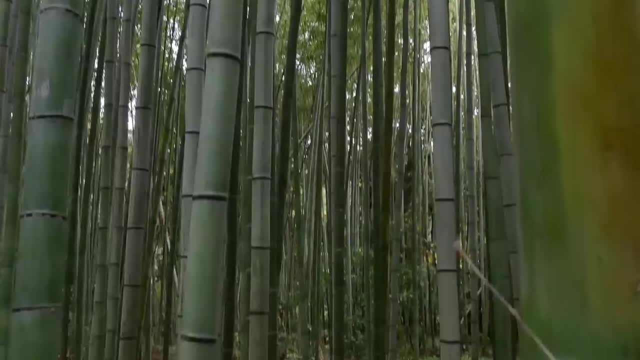 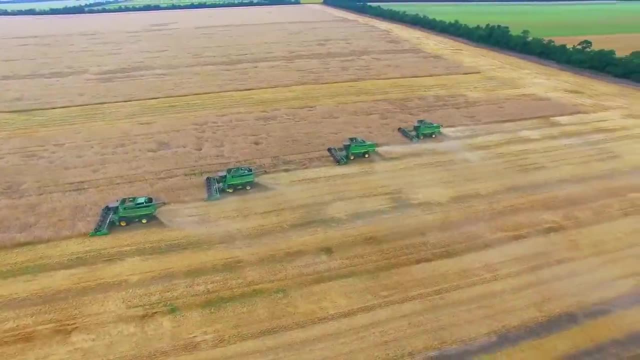 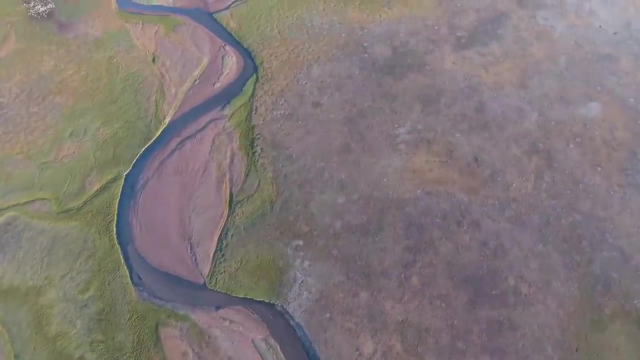 grasses have colonized every patch of soil, from tropical to temperate forests, savannah to steppe scrubland to desert. Humans have taken these grasses and shaped them over generations into crops that feed the world. today. Their homelands are the seeds of grass we call 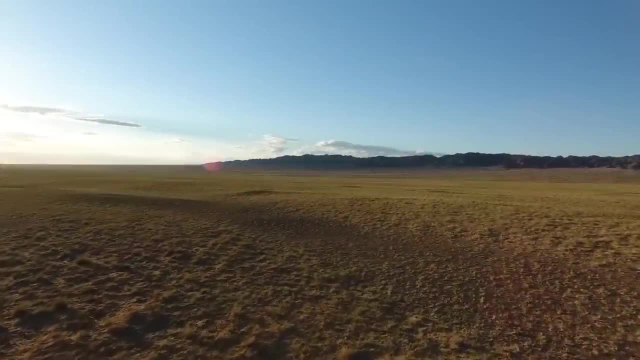 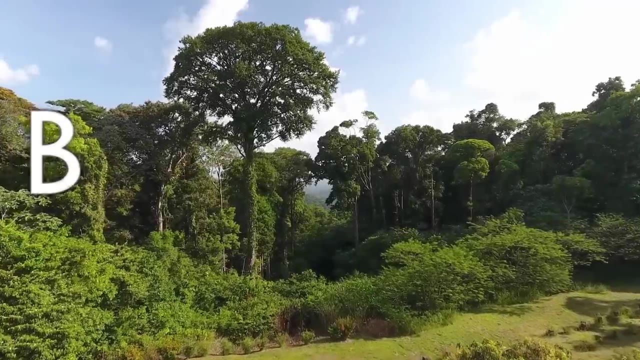 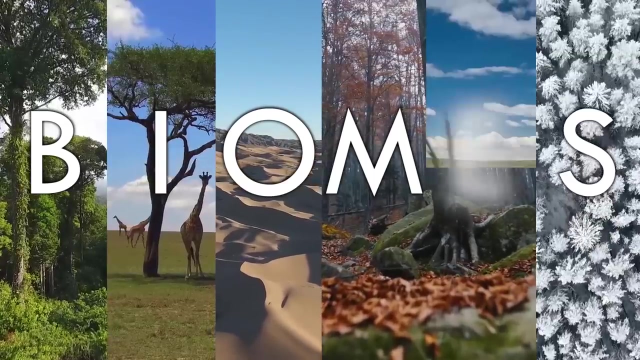 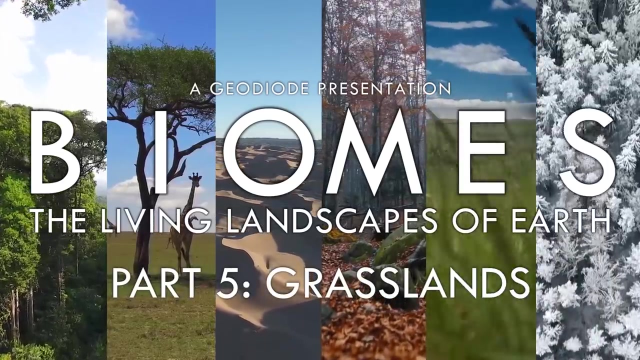 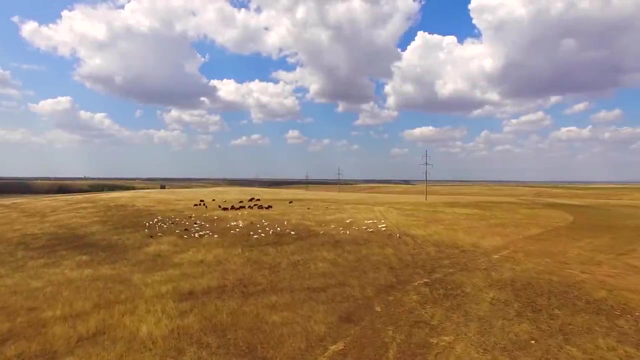 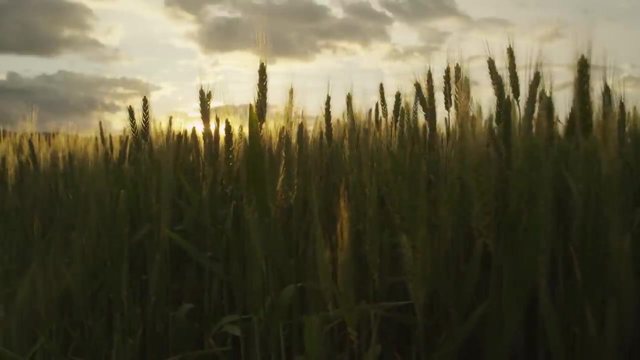 meadow, prairie, pampas, veldt and steppe, The world's grasslands. Grasslands are one of only two biomes on our planet to be completely dominated by a single plant. But what is grass? A simple definition is a non-woody plant. 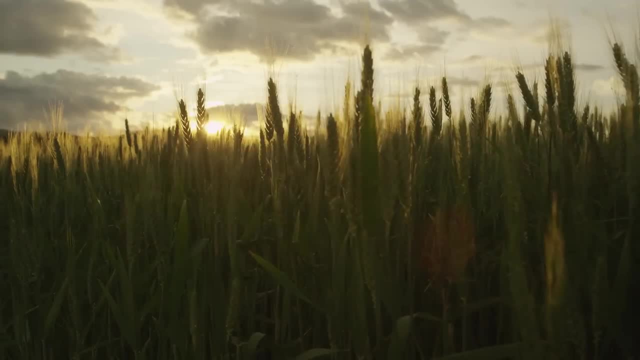 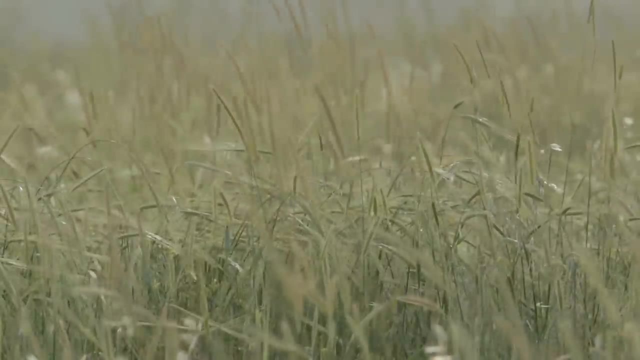 containing a hollow stem for strength, bladed leaves for photosynthesis and a flowering bundled seed head for reproduction. This simple but highly successful formula has evolved since the end of the Cretaceous period about 66 million years ago to form over 12,000 species today. 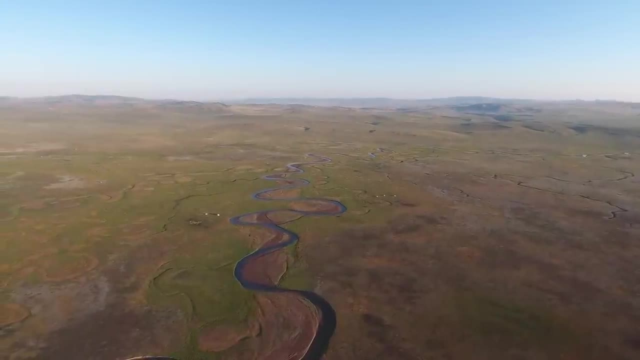